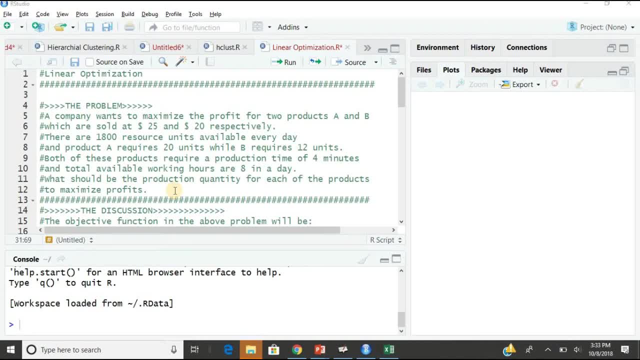 What is your objective function and what is your constraint? So objective function is to maximize profit. Constraint is: I have two constraints in this condition, Like I have 1800 units of resources per day And I have four minutes for each product, Or each product requires, 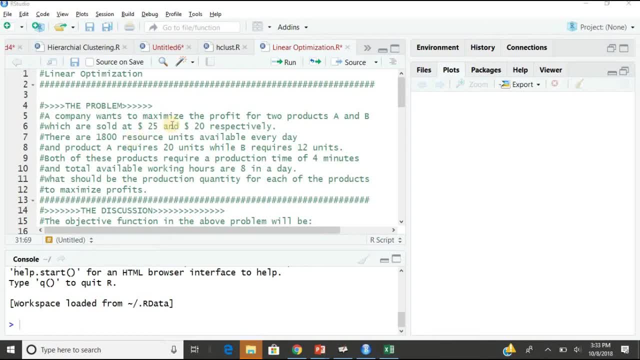 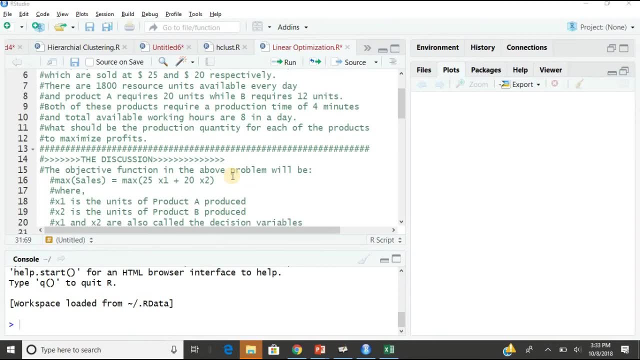 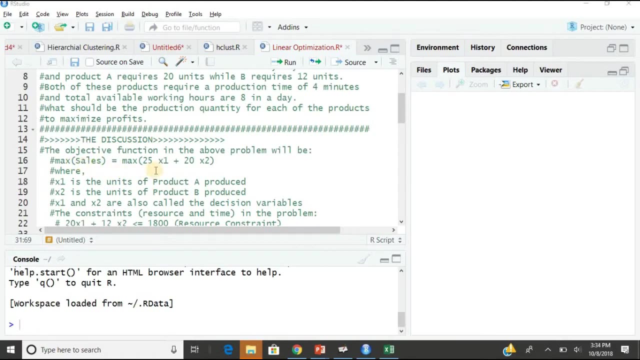 four minutes for production. These are the two constraints, And we are working eight hours in a day. Fine, Now let us see. This is a basic calculation that all of us know. What we are trying to do is we have to maximize the sales, That is, we have to find maximum of these two, Like: if x1 is the units of 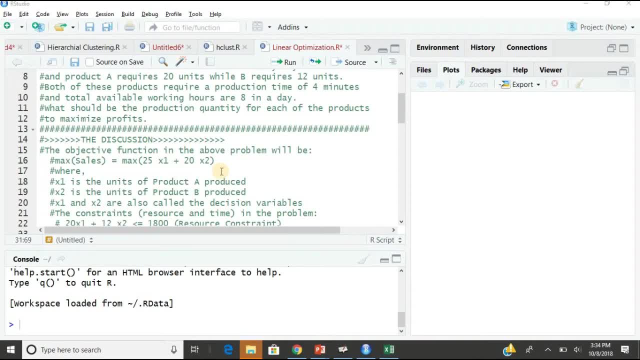 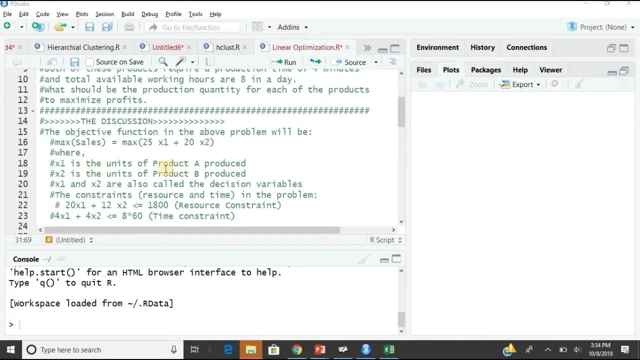 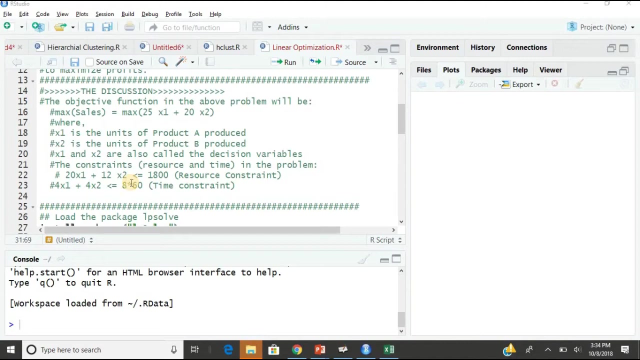 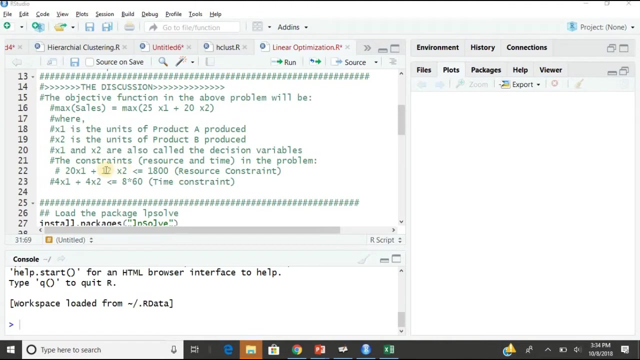 production of A. x2 is the units of production of B. We have to maximize that. That is my objective. x2 is the units produced for B. So now see, now we have the constraints, And this is what I explained you in the Excel also. 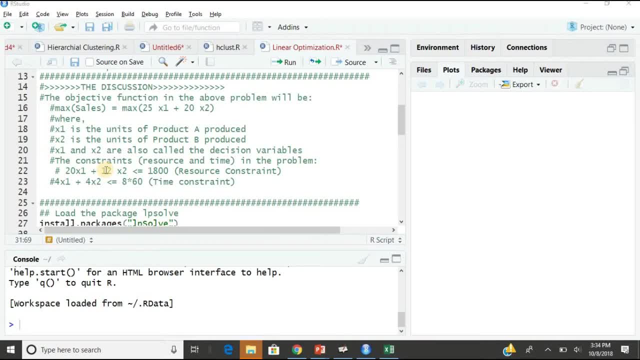 Okay, In Excel we actually what we modeled the entire thing. So what we did was actually mathematically this: Okay. So these are the resources. That is, 20 units, Okay, 20 into 1 plus 12 into 2.. That is giving me 1800 resources And at the same time, like 400 and 400, 4 minutes. 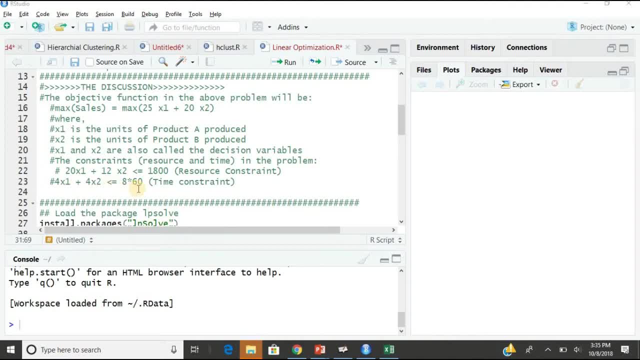 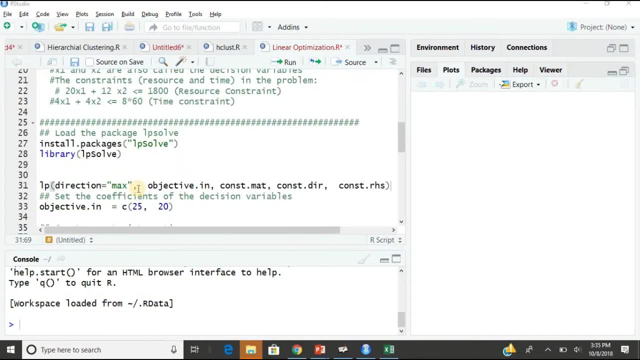 for the first one and 4 minutes for the second one. That is, 8 into 16.. Okay, So these are the constraints we are working upon. So I hope you have installed the package. We will be requiring the package LPSolve And if you have installed that, we can put it in library. And before moving ahead, okay. 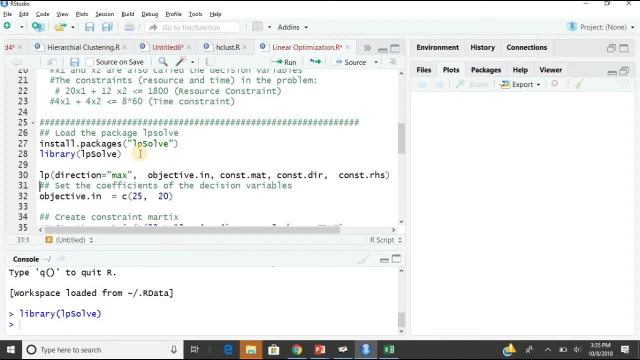 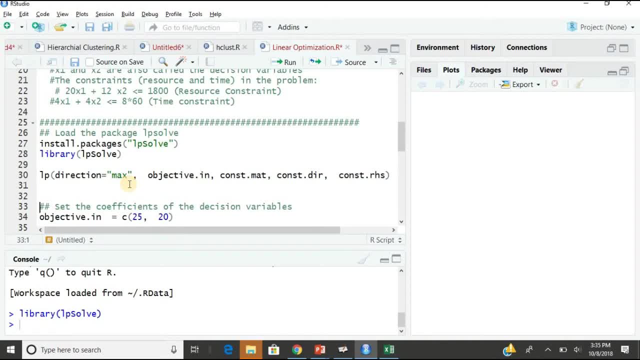 The LP function. it will require, Okay, will require certain arguments, and once you, you know, create those arguments. it is very simple. so, if you see, i will require one, two, three, four and five things. this is the basic argument that will require for the function. okay, one is the direction. okay, direction means nothing but max. 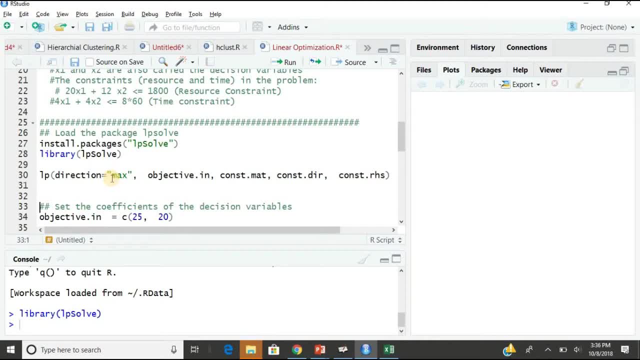 and min. this is what we saw in excel. okay, what is the objective set to? we said max, we click over max. so here that same thing is direction, max or min. don't go double quotes, okay. so if it is a minimizing problem, i will say: direction equals to min, getting the point. so your direction, okay, and 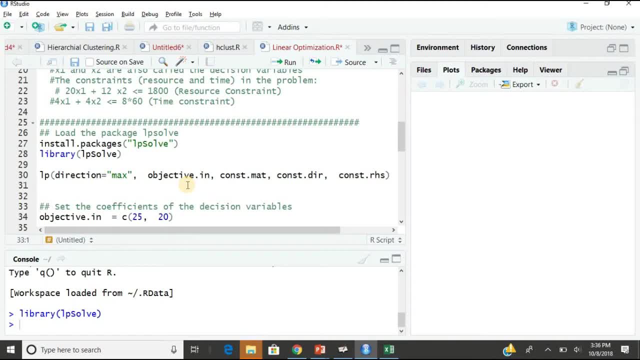 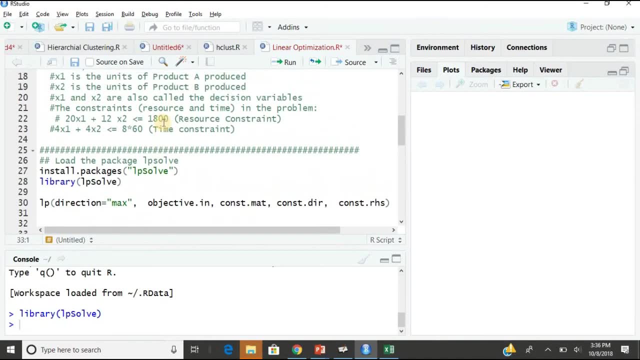 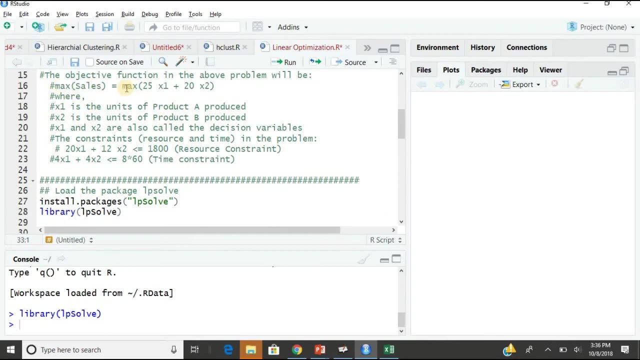 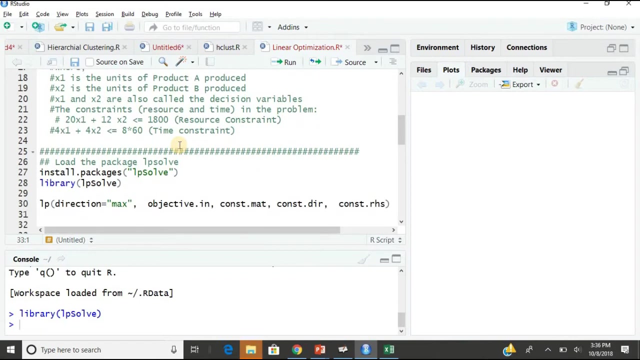 then you have to create a function for your objective object. okay, something equals to: okay, we have created the object objective. like you see, like this is my objective function. okay, so you have to create an object for this. okay, so create an object for your object function. that is number two direction. we have decided here: max min. number two: your object, okay, objective. 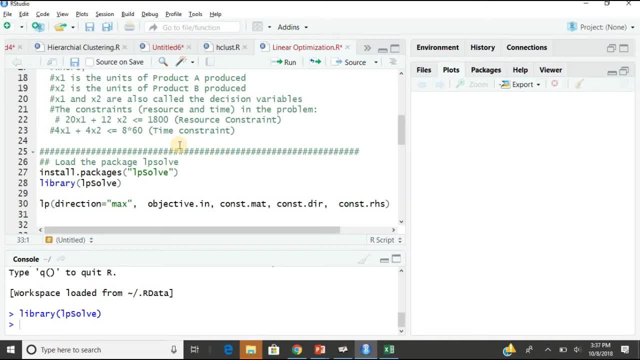 camera key. i have to maximize the profit. okay, like 25 into x and plus 20 into y. that is my object, okay, and then your constant matrix, a constraint matrix, things like c capacity, what course is psm, tens? and 2 by x, c, this is the millennial. 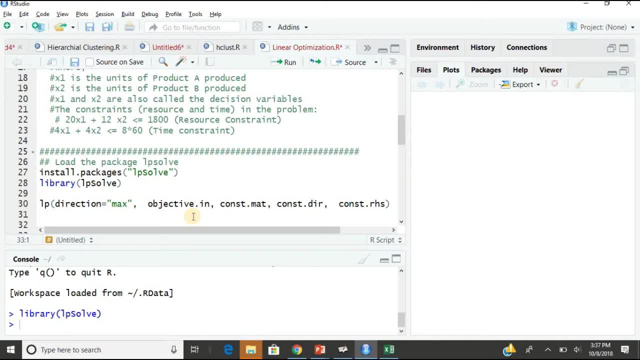 okay, of different objects in which some data will be stored, but you have to create them separately. okay, first i'll explain syntax. okay, so i'll require five arguments. first argument: your direction. Second argument is your objective. and third object is your constraints. You have to make a matrix of constraints. 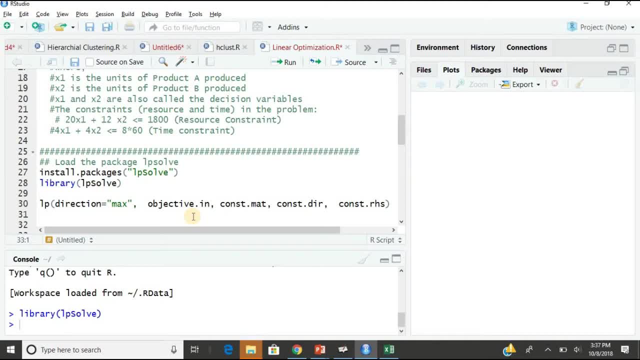 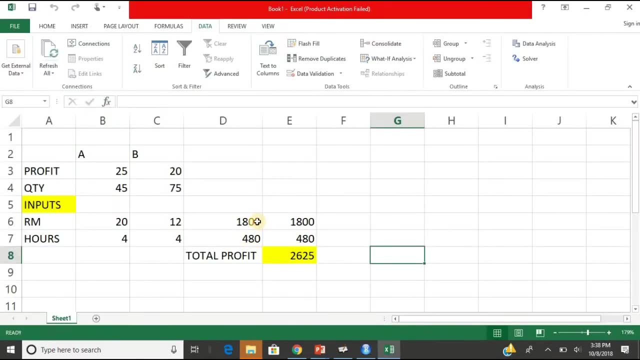 Whatever your constraints are like, we have made a table of constraints in excel. The same thing you have to- or you can see, this is what your constraint matrix Getting the point. This should be less than equal to this. this should be less than equal to this. 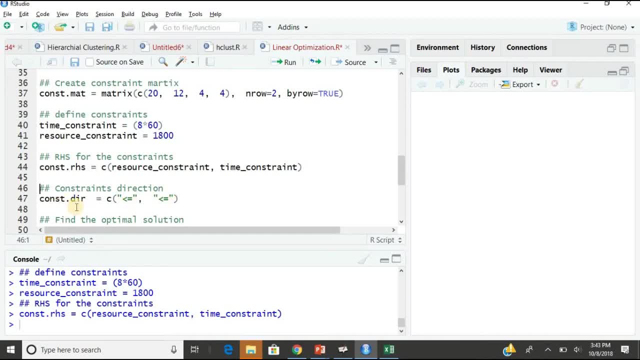 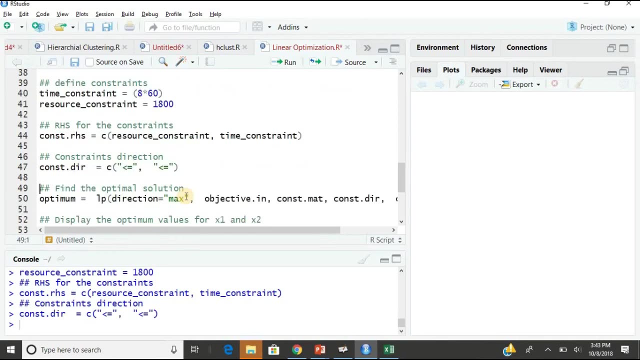 RHS. Okay, And then constraint direction. I have two constraints: time constraint and resource constraint. In both of them, the direction is less than equal to. okay. In both the cases, the direction is less than equal to. So just put that: yeah, less than equal to. so now, finally, the same thing. okay. 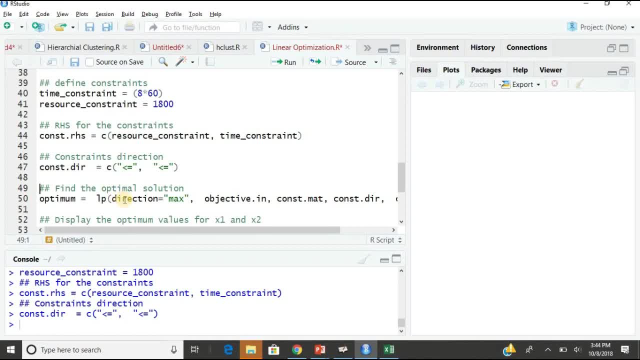 Now I'm just writing an object called optimum and I'm writing the same command, the syntax that I showed you in the beginning. Okay, The command that I showed you in the beginning is the same, just okay. now I have created that. 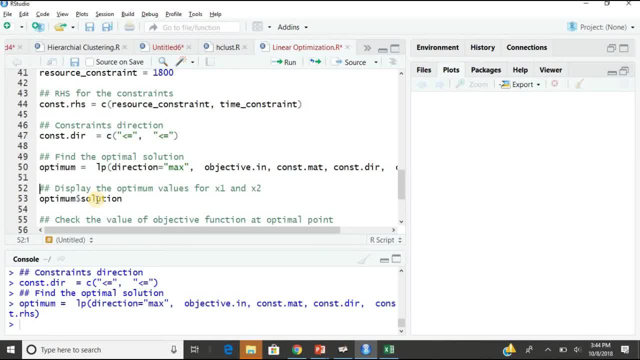 Fine, Now see, now the object has become your optimum. Now display the optimum values of x1 and x2, means how many units of A and how many units of. so optimum dollar solution. If you see, just if you, you know, just run optimum, you'll see, you'll get a huge output. 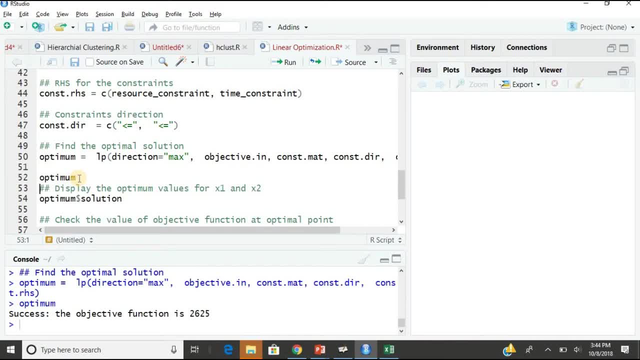 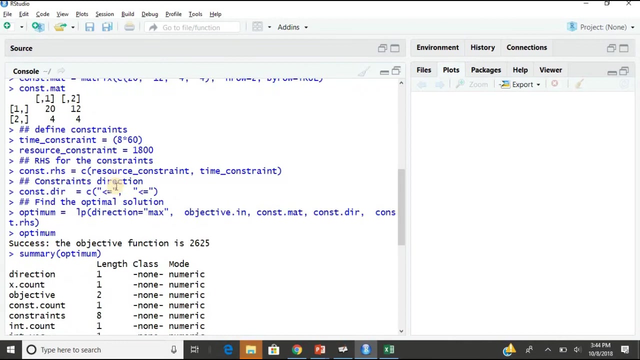 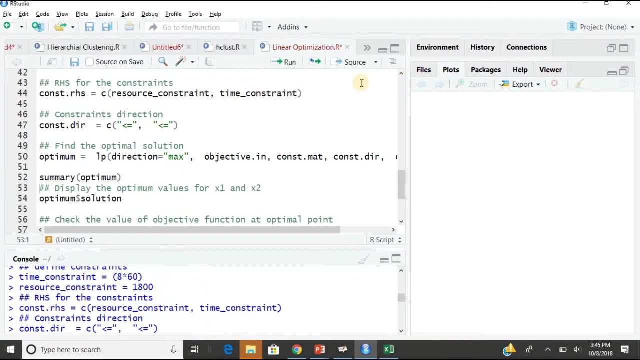 Okay, Just sorry if I say summary and optimum. you see, I get lot of output okay, in which I have direction, x, count, objective, lot of things. Okay, I'm not worried about all those things. Let us see first, one by one. 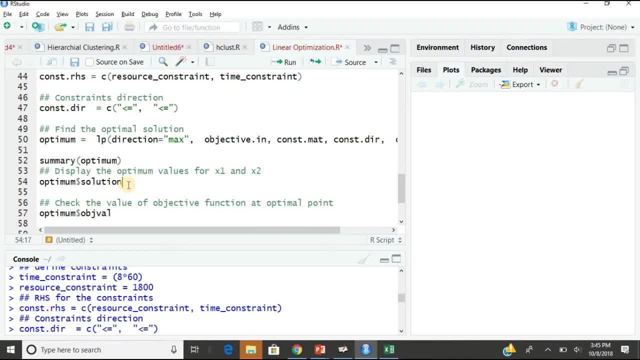 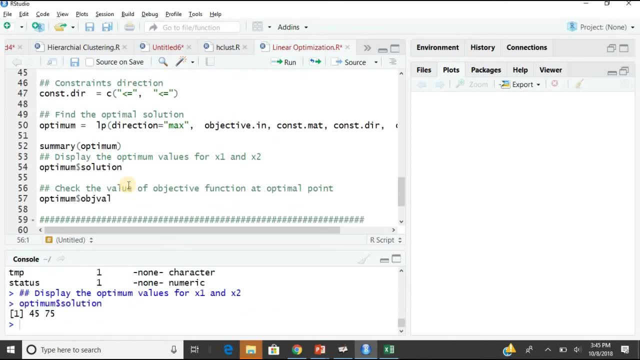 So if you put optimum dollar solution, it will give you how many values. this is what I wanted to find, right, See how many units of A, how many units of B to be produced. So just write this. So it says 45 units of A and 75 units of B to be produced, straight forward. 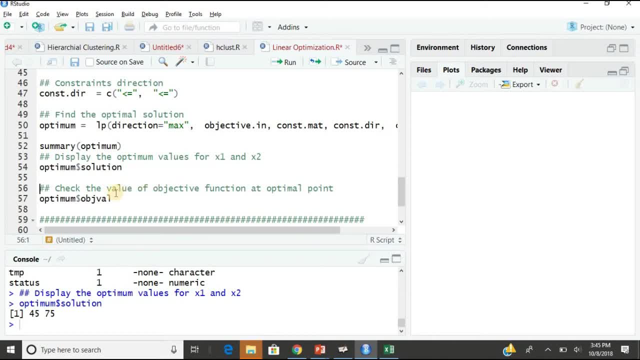 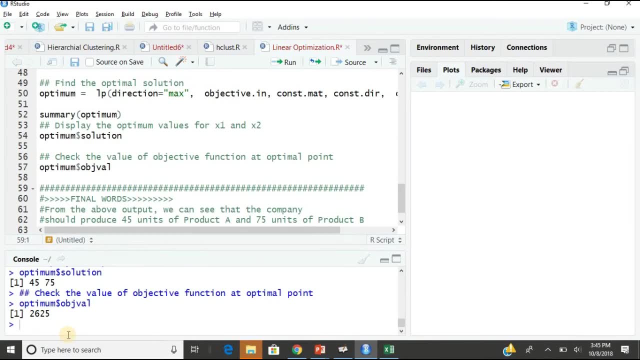 Okay. And then it says: check the value of objective. So optimum objective value: 2625 units. Okay, 2625 units to be. this is the objective. that is total profit. Okay, This is the maximized profit that I have. 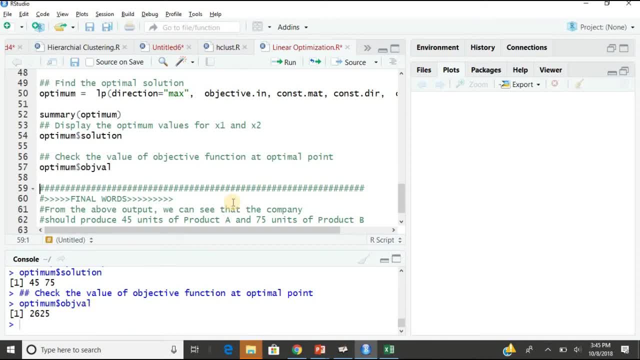 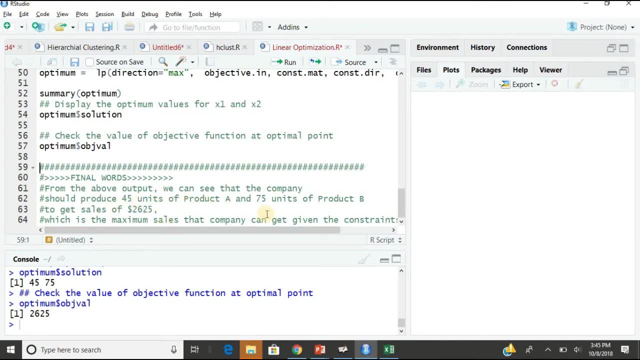 So what is the final conclusion from this? whatever we have done till now, that is, from the above output, we can see that the company should produce 45 units of product A, 75 units of B to get a sales of dollar 2625. 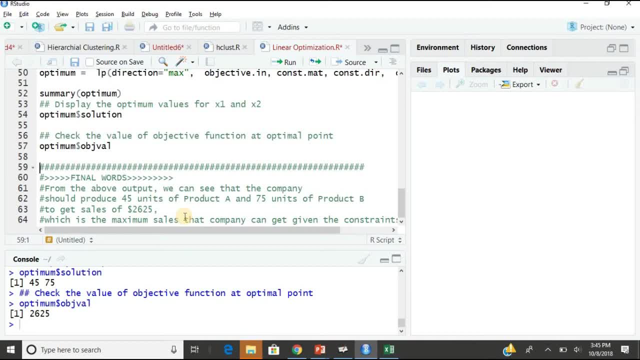 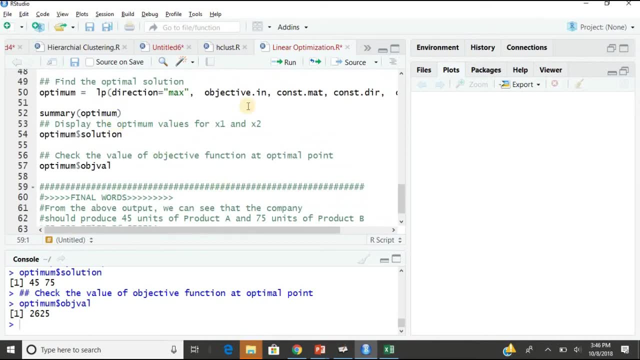 Fine. So we have solved the same problem using Excel. We have used R also to solve the problem. We have used R also to solve it. Very simple, What you have to simply remember is this syntax: okay, The syntax of LP, direction max: okay. 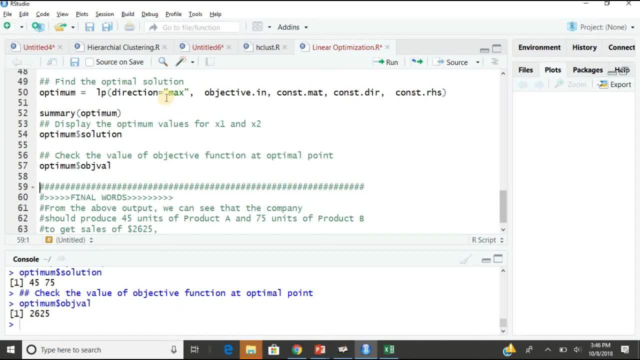 If it is a minimized problem, I will say: direction min. okay. Objective dot in. that is the objective here. it was maximizing the profit. So you create an object dot in C the profit contribution by A, profit contribution by B. Fine, 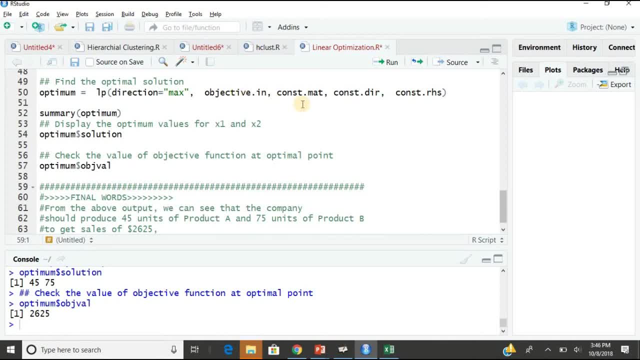 Okay, And you have constant matrix, constraint matrix, So whatever the constraints, you have, put them in a matrix. Okay, So that constraint matrix will come. Sorry, It will be on UMS, I don't remember the date. 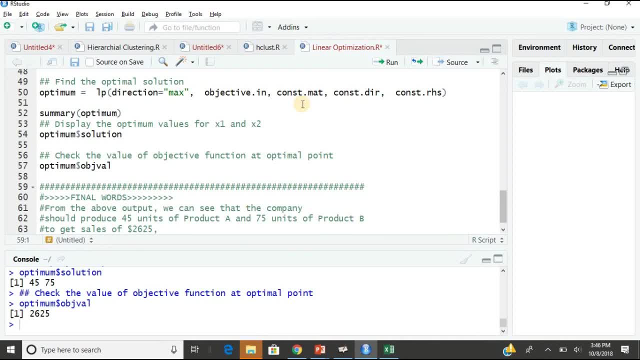 I think 30th, 30. I think just check, check the UMS. Okay, Fine, Okay, Constraint direction. What is constraint direction? Some final value was given. I have 1800 units. So whatever the constraint is, it should be less than equal to 1800.. So in both cases, less than equal to And constraint RHS: this object has all the values stored in it. That is time constraint and resource constraint. That is saved in it.